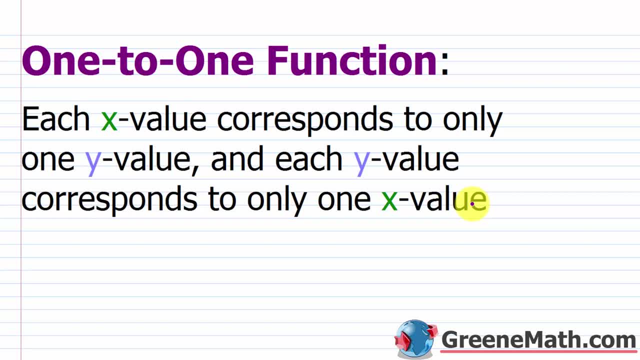 line, the y value is always the same. So if that horizontal line representing that kind of single y value impacts the graph in more than one location, that function is not going to be a one-to-one function. So if that horizontal line is not going to be a one-to-one function, 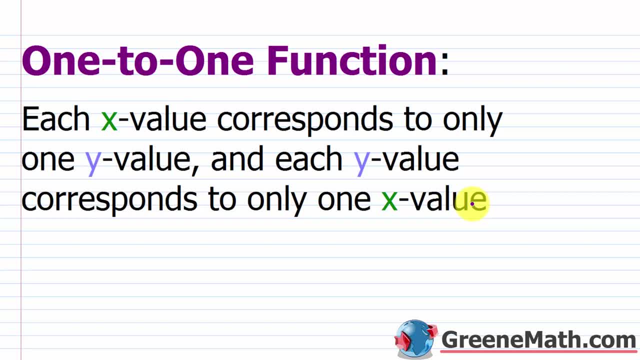 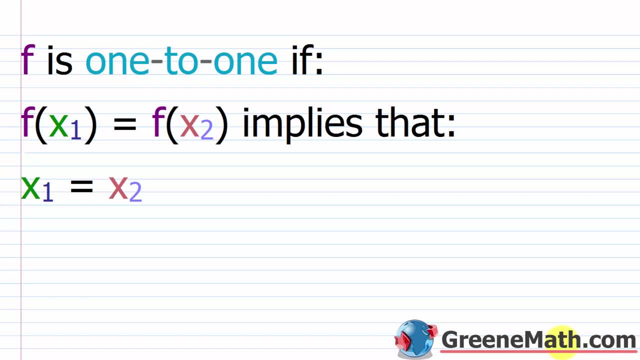 because that single y value is associated with more than one x value. Now, additionally, we have an algebraic method that we can use. In some cases this is faster. In some cases it gets a bit complex, So it just depends on the given scenario. But if you're in a pre-calculus course or college, 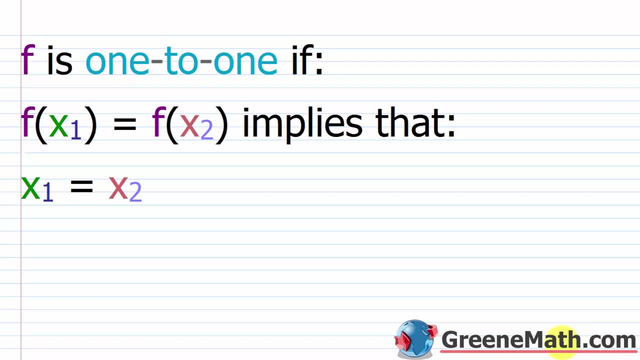 algebra course. a lot of times they'll tell you that you need to show this algebraically and they'll give you reasonable examples to work on. All right, so this is what we want to start with here. It's just basically breaking the definition of a function. So if you're in a pre-calculus course, 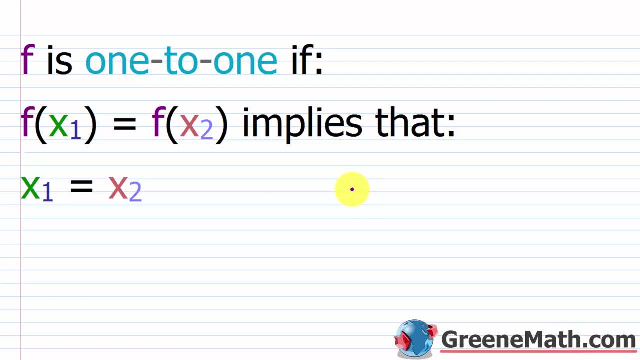 it's just basically breaking down the definition we just saw, but into a more kind of algebraic format. So f is said to be one-to-one if, and only if, f of x sub 1 is equal to f of x sub 2 implies that x sub 1 equals x sub 2.. So what does this mean? If you read this in your textbook, you 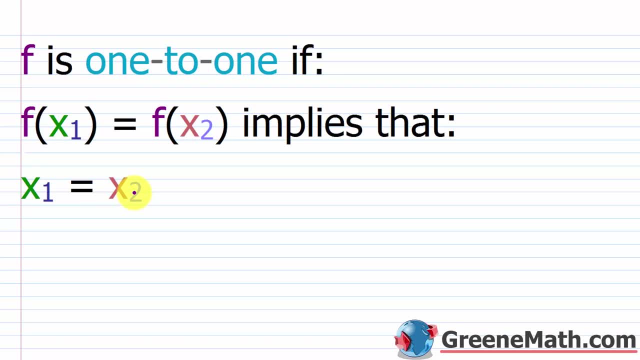 might get confused by it. The only thing you need to focus on is the fact that when we have f of x, it doesn't matter. this is f of x sub 1.. f of x in general is what. It's, just a replacement. 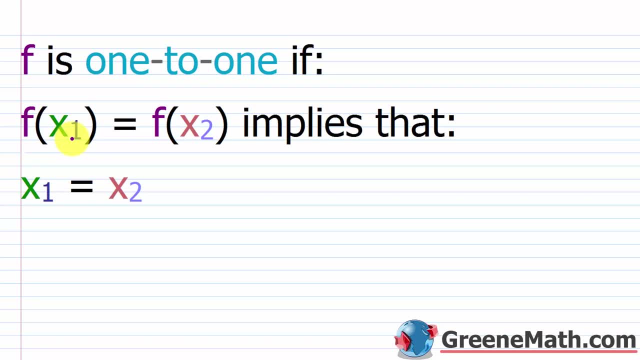 For our variable y that we're so used to right, it's the output of a function. So f of x sub 1 is just the output. when I plug in the x sub 1 for each occurrence of x in that function, It's the. 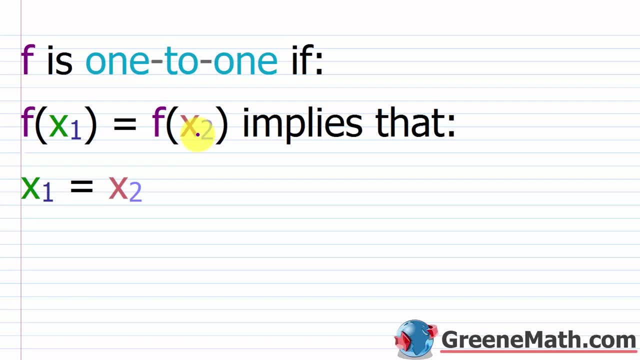 same thing for f of x sub 2.. It's just the output, or again the y value when I plug in x sub 2 for each occurrence of x in the function. Now, if these two y values are equal or the same, well, if the 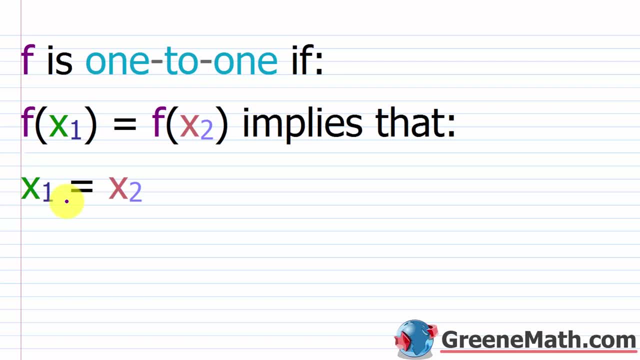 y values are equal or the same, well then, the y value is the same. So that's all this notation is really saying here. It's written in a format that is confusing, but once you kind of break it down it's not so bad. So what I want to do now is just show you a method that relies on this kind of. 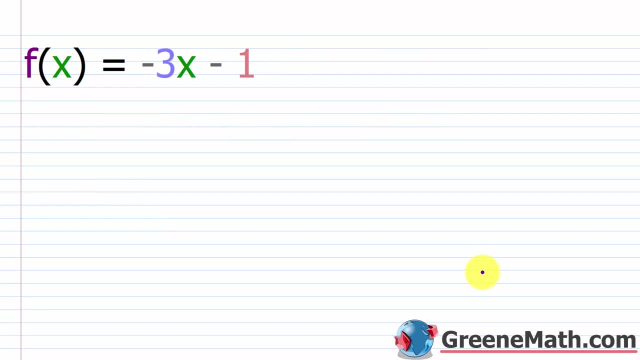 notation here and basically we'll just jump right into an example: What you want to do if we have f of x equals negative 3x minus 1, you want to say, okay, if I had f of, you can use x sub 1.. I'm going. 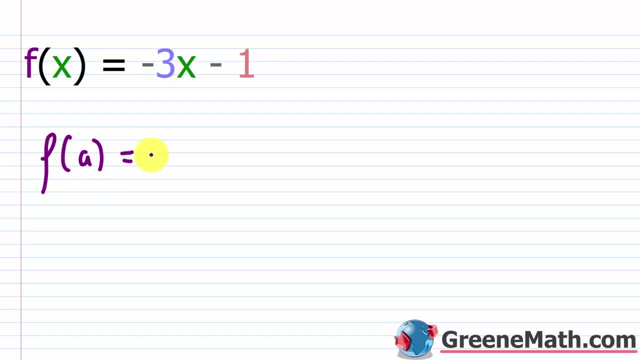 to use a and b here. so I'm going to say f of x sub 1 is equal to negative 3x minus 1.. So I'm going to say f of a, this is negative 3a minus 1.. All I did here was I plugged in an a where there was an x. 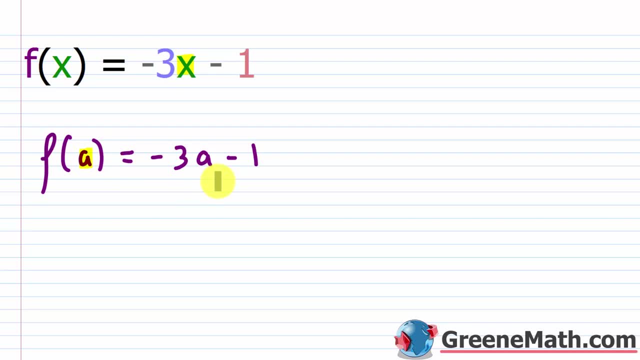 here. Okay, that's all we've done, and we've seen this before in previous lessons. Now, what I also want to do is I want to look at f of b. So what would that be? So it would be negative 3b minus 1.. 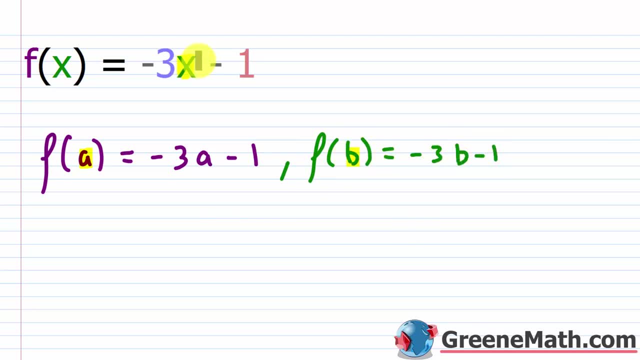 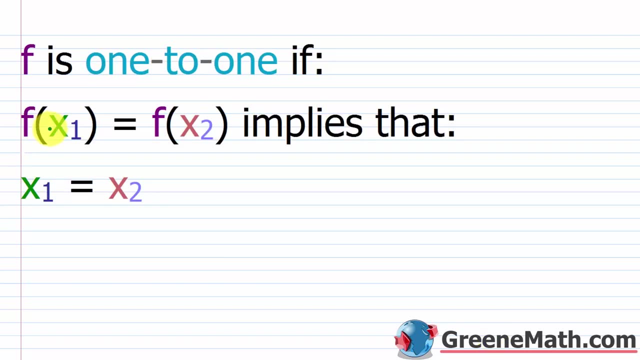 Again, all I did was I plugged in a b where there was an x in that function. Okay, so so far, so good. So from our notation let's just go back to it again. we have: f of x sub 1 is equal to f of x sub 2 implies that 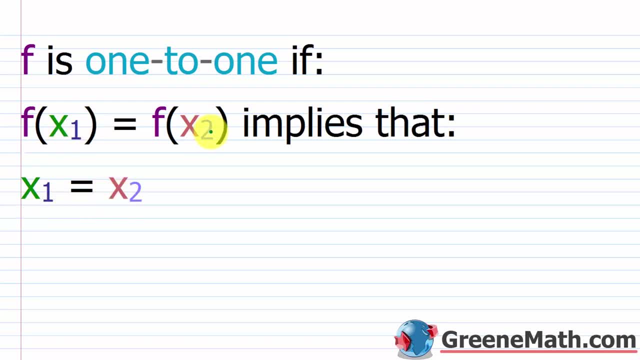 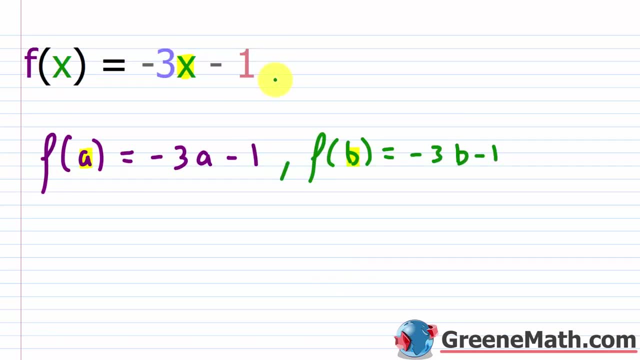 x sub 1 equals x sub 2.. Well, instead of using x sub 1 and x sub 2, we're using a and b, just to keep it simpler, And so what I want to do here is say: okay, if it's true that f of a is equal to f of b. 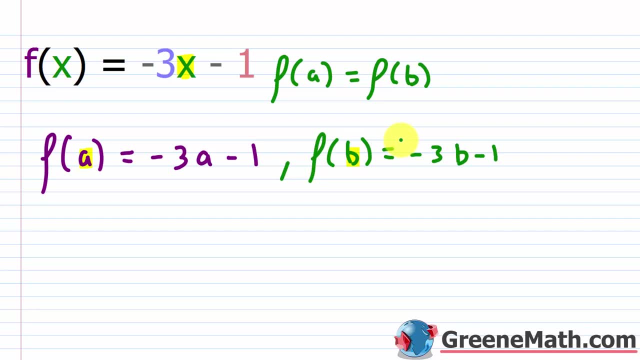 okay, then it has to be the case that a is equal to b. okay, otherwise this function is not going to be true. So what we can do is we can set these two equal to each other. Remember, f of a is actually equal to this and f of b is actually equal to this. Okay, so what I'm going to do is I'm going 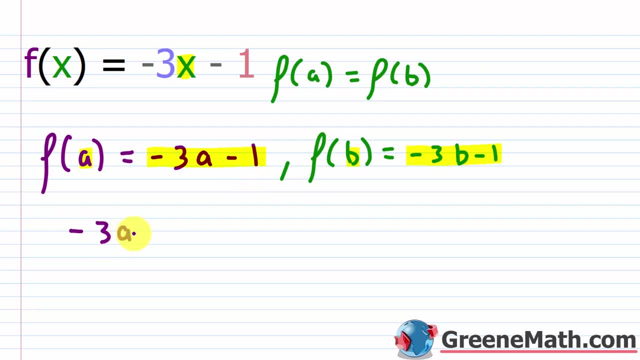 to set these two equal to each other. So I'm going to say negative 3a minus 1 is equal to negative 3b minus 1, and if it's a one-to-one function, it should be true that a is equal to b. 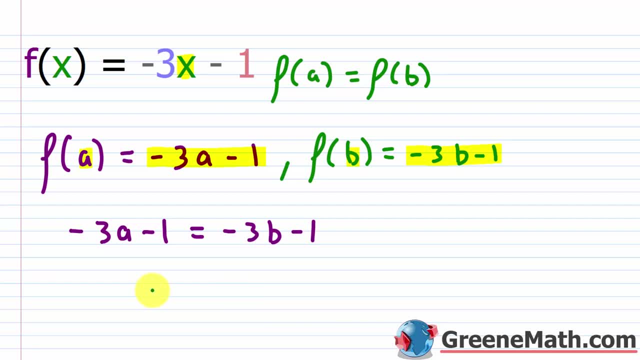 always. So let's go through and kind of simplify. this is really simple. We're just going to simply run through this and we're going to set these two equal to each other to. you could say you're solving for a. you could say you're solving for b, i'm just going to go. 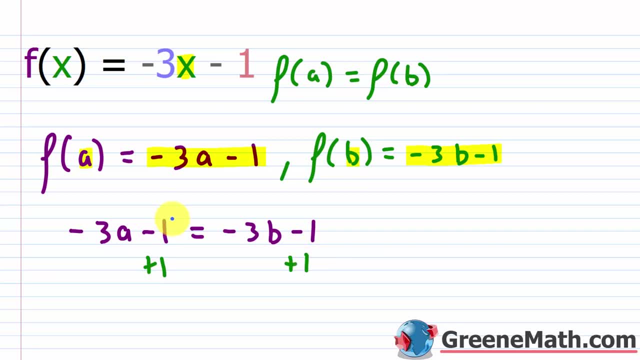 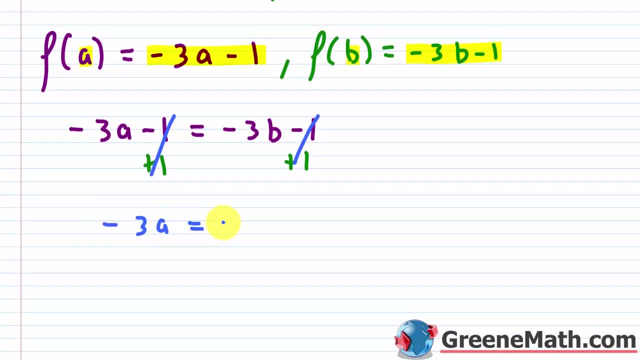 through and add one to both sides, and what i'm going to do here is i'm just going to cancel this, and that's going to give us what- let me kind of scroll down a little bit- that's going to give us? negative 3a is equal to negative 3b. if i divide both sides by negative 3, what am i going to get? 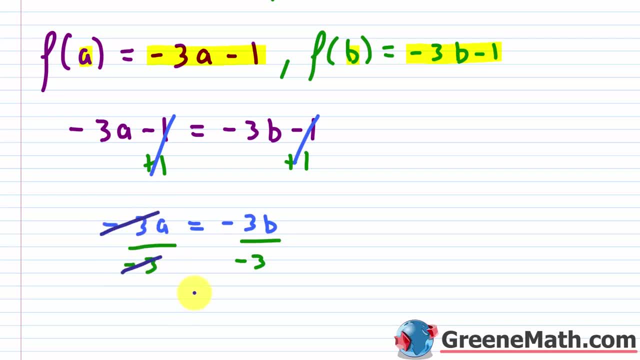 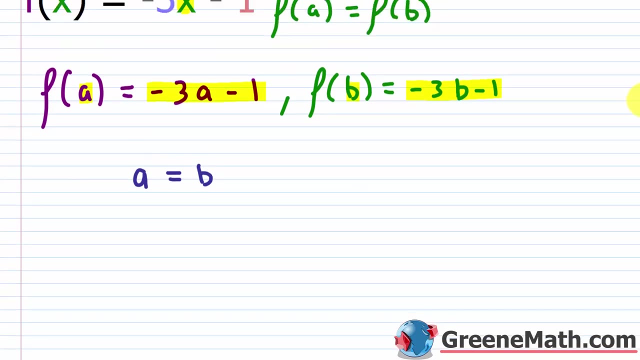 well, we know that this is going to cancel with this and this is going to cancel with this. so i get that a is equal to b, so we've proved that this function is one to one. let me erase this real quick and let me just drag this up here and let me just go back up so we can recap this real. 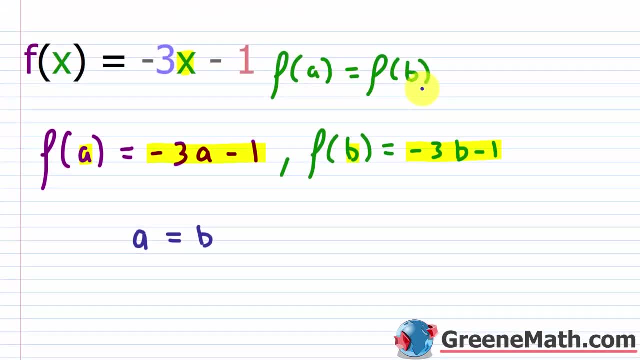 quick. we said that again. if f of a is equal to f of b and this function is one to one, then it has to be true that a equals b. well, we have f of a defined as negative 3a minus 1. we have f of b. 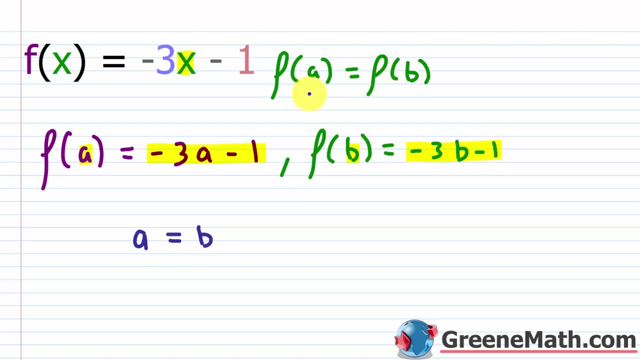 defined as negative, 3b minus 1. so if i set these two equal to each other, you get that a is equal to b. so we've proved that this function is one to one. let me erase this real and I go through a process of either- you could say I'm trying to solve for a- or b, doesn't really. 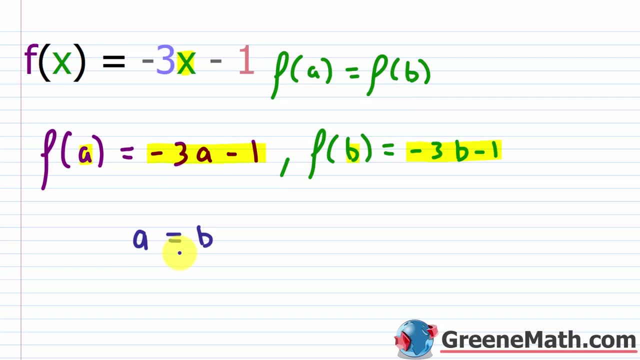 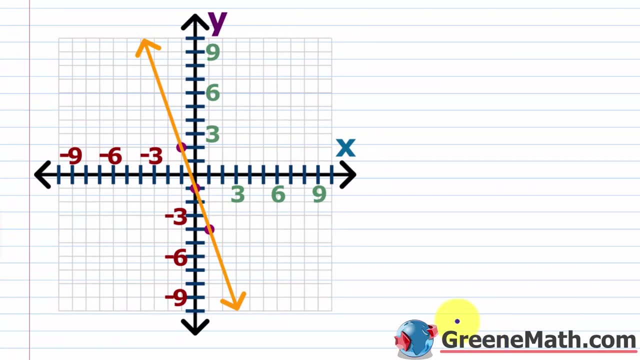 matter. I end up with this: a equals b, So I know this function is one to one. Now, if you want to look at a graph of this guy again, I don't have to draw horizontal lines here- you can see that. 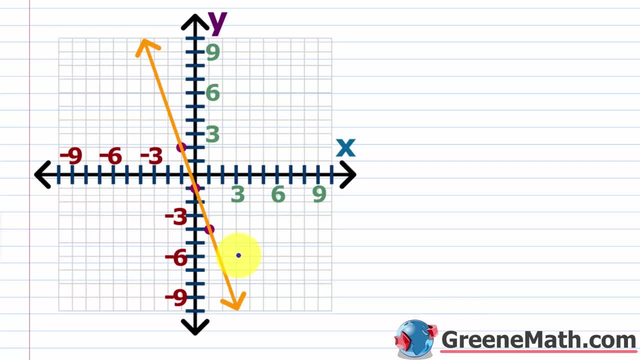 this graph. here there's no horizontal line that would impact it in more than one location, So we know that this function is going to be one to one when you first start doing this. if you want to graph it to check and make sure that you got the right answer, that's probably a good idea. 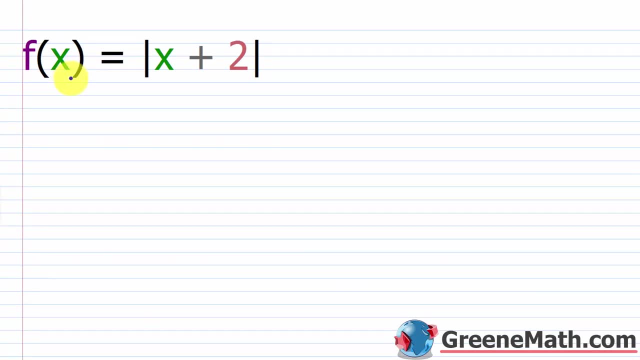 All right, let's look at another example. So we have f of x equals the absolute value of x plus two. Again, if I use f of a, this is what just plug in an a where there's an x. that's all you. 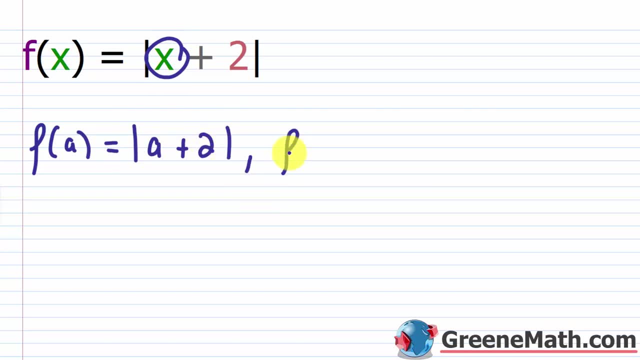 have to do So. a plus two then for f of b. okay, I'm just going to now plug in a b where there's an x, So we'd have b plus two. nothing that's too fancy, nothing that's too confusing Again. 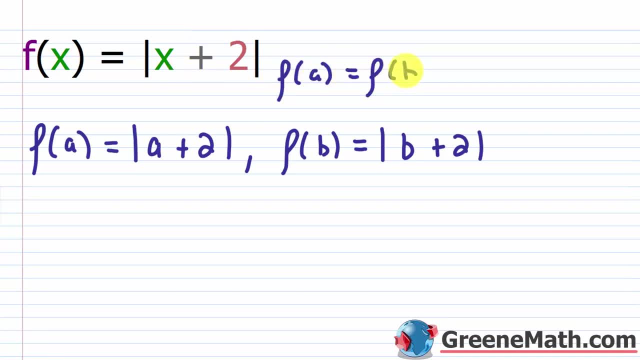 if f of a is equal to f of b, then it's got to be true that a equals b, and that's got to be true all the time. So what can we do here? Again, this is f of a, this is f of b. So if these two are, 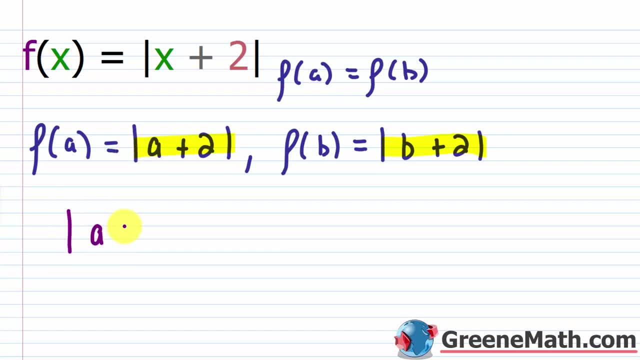 equal. set them equal to each other. And let's see. So we have: the absolute value of a plus two is equal to the absolute value of b plus two. Now we've solved absolute value equations before And we know that if we have an absolute value expression equal to another, 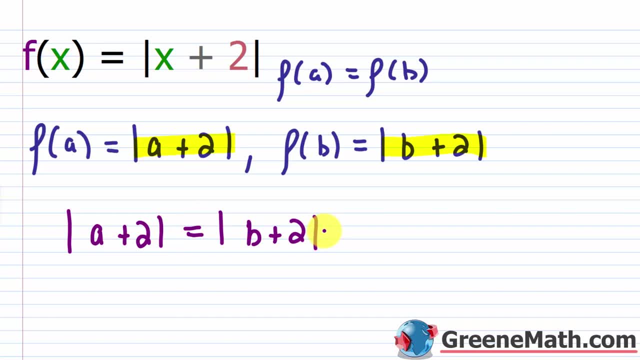 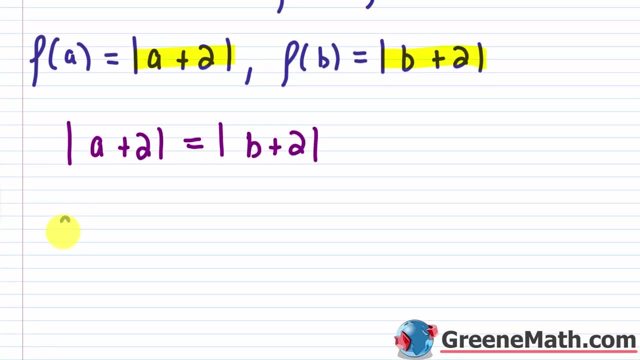 absolute value expression. well, these two can only be equal if- what The first scenario is- you drop the absolute value bars. So the first scenario would just be: a plus two is equal to b plus two. But because you have absolute value involved here, there's going to be an or right. 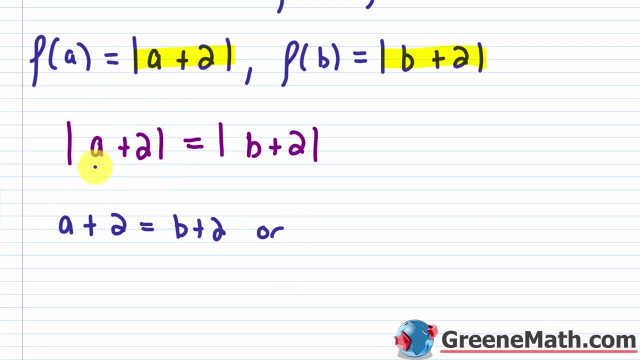 So it could be also be true that the negative of one of these expressions is equal to one of the expressions. So in other words, I would drop the absolute value bars, So I put a plus two is equal to b plus two, And then I would wrap one of these in parentheses, it doesn't matter which. 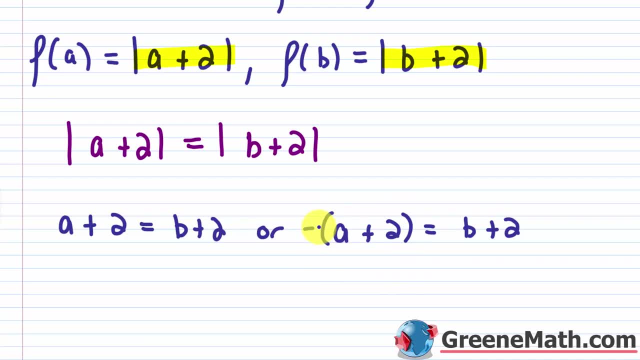 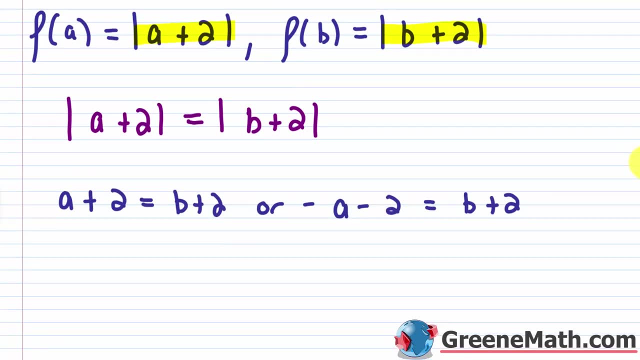 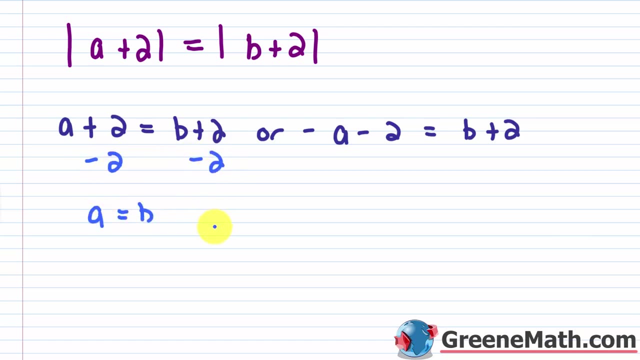 one and I would put a negative sign out in front. Now you can distribute that and say: this is negative a minus two, And what's going to happen is you're going to run into a problem. okay, So over here it's fine. I subtract two away from each side and I get: a is equal to b, But this: 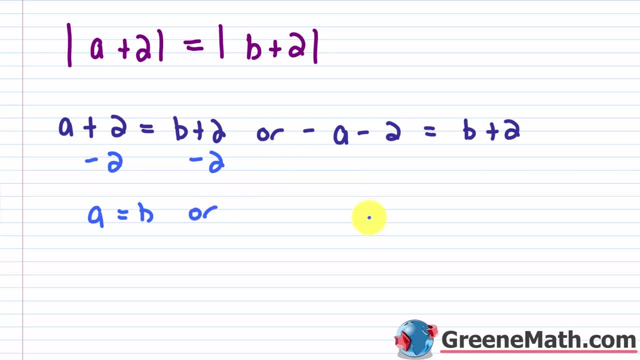 is where it gets messed up, because you have this or, and over here I have negative. a minus two equals b plus two, And I get a is equal to b, And I get a is equal to b, And I get a is equal to b. 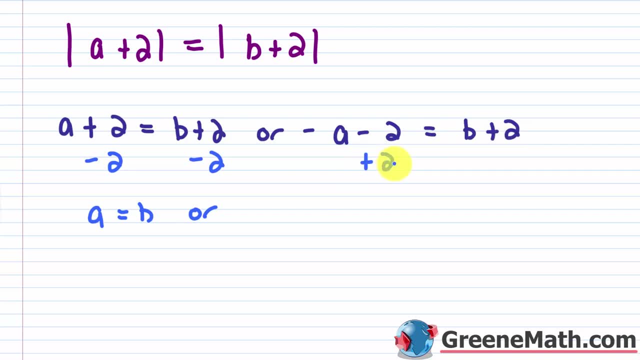 Let's just solve it for a. So in that particular case I would add two to both sides And I would have negative. a is equal to this: cancels b plus four, And then to get a by itself, let's divide: 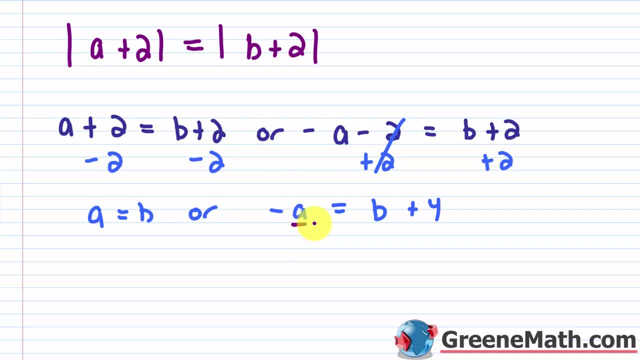 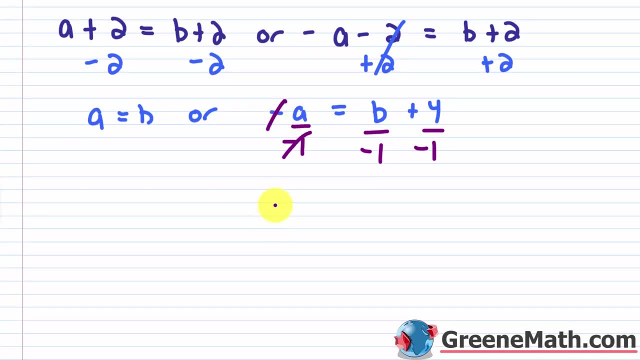 both sides by negative one, or you could multiply by negative one, it doesn't matter. So let's divide both sides by negative one And let me scroll down and get a little bit more room. So we know that this is going to cancel And I'll have. a is equal to negative b minus four. Now the problem lies. 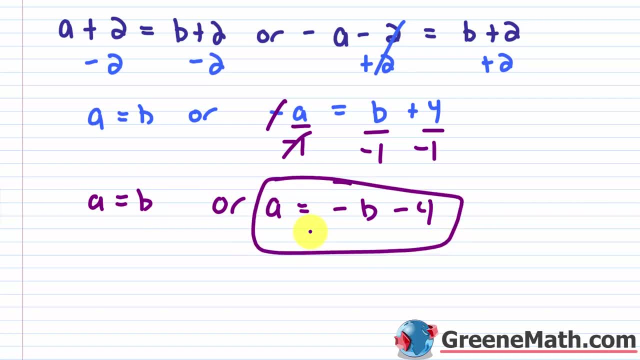 in this one right here, okay, it's okay. this one right here on the left is fine, But you have this or situation And that's what throws a wrench in this. So this function is not going to be one to one. So let's look at this graphically And we can clearly see this function is not one to one, If I 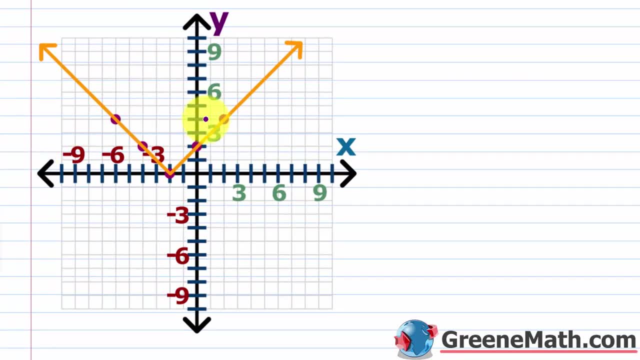 drew a horizontal line through. if I go up to y equals four. so let's say I had a horizontal line, y equals four. let's just draw that in real quick And not perfectly straight, but you get the idea. And when I look at this guy again, it's going to impact the graph here and also here. So that's an. 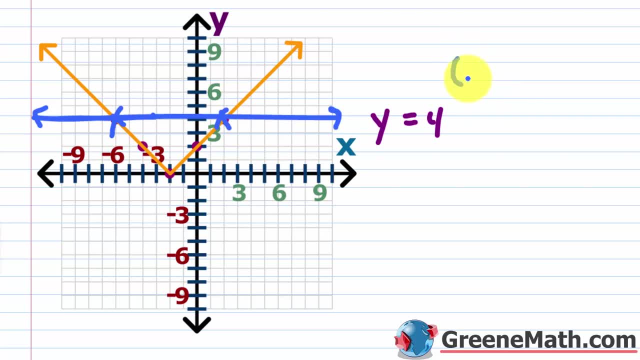 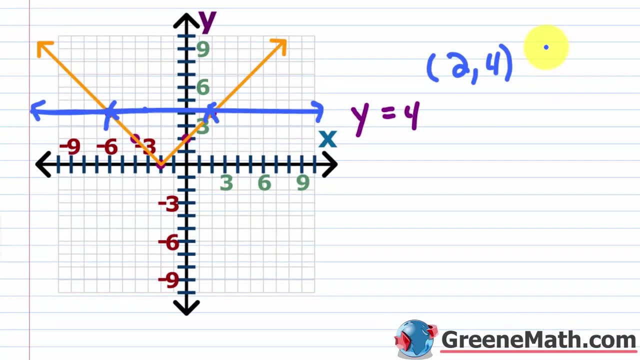 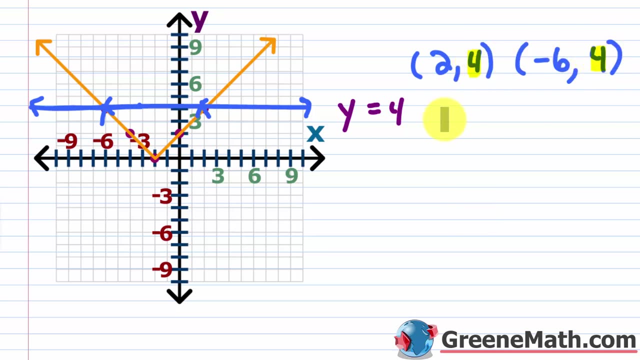 x value of two and a y value of four. So two comma, four works. and then also an x value of negative six and a y value of four, So an x value of negative six and a y value of four. So this y value of four is associated with two different x values, two and negative six. So of course, 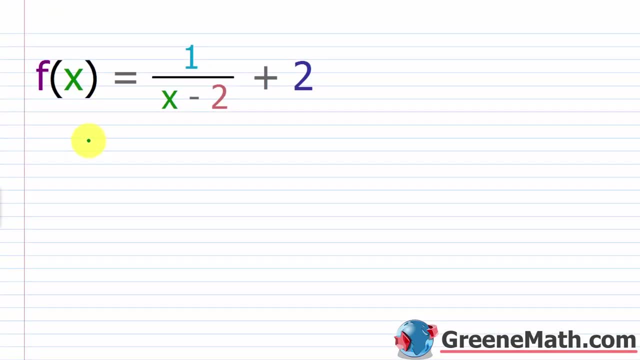 this is not a one to one function. Alright, let's take a look at another one. So now we have f of x equals, we have one over x, minus two and then plus two. So again I'm going to go: f of A is equal to one over A, minus two, then plus two. then I'm going to do: f of B is equal to one. 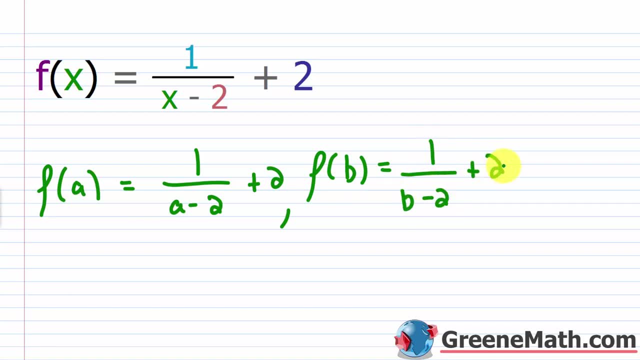 over B minus two and then plus two. Okay, so again, what I want to do is set these two equal to each other. So this is f of A, this is f of B. set them equal to each other and show that a. 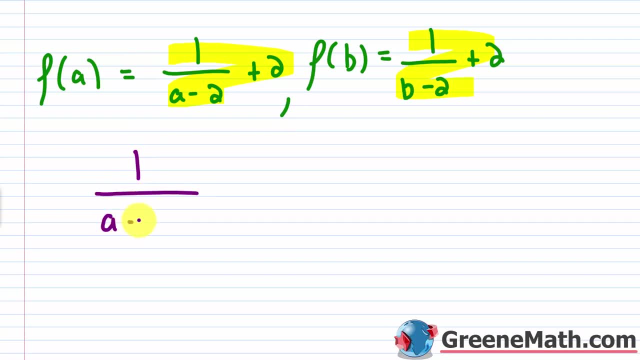 1 to 1.. So 1 over a minus 2 plus 2 is equal to 1 over b minus 2 plus 2.. Well, I have 2 on each side, so I can just get rid of that right if I subtract 2 away from this side and I subtract 2 away from. 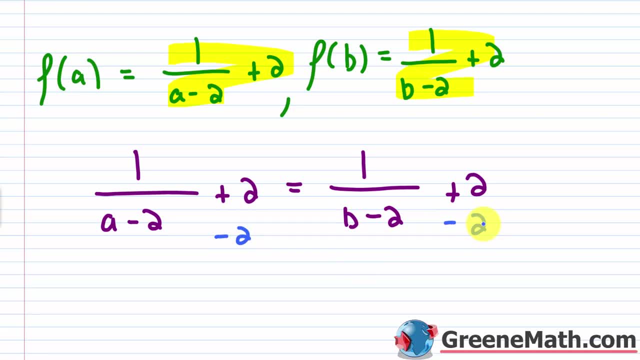 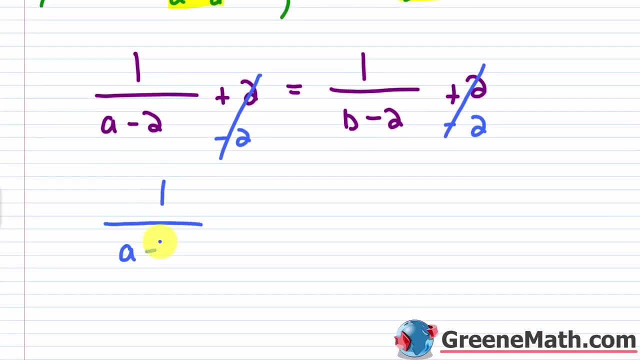 that side. I'm just subtracting the same thing away from both sides of the equation, so it's going to cancel over here and cancel over here. So let's scroll down now and what we have is 1 over a minus 2 is equal to 1 over b minus 2.. So the quickest way to solve this is just to cross. 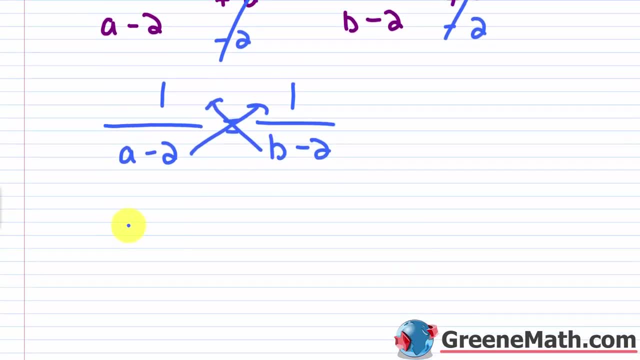 multiply. okay, so what we would have is what we would have: b minus 2 times 1, which is just b minus 2, is equal to a minus 2 times 1, which is just a minus 2, and of course now I can just add 2 to. 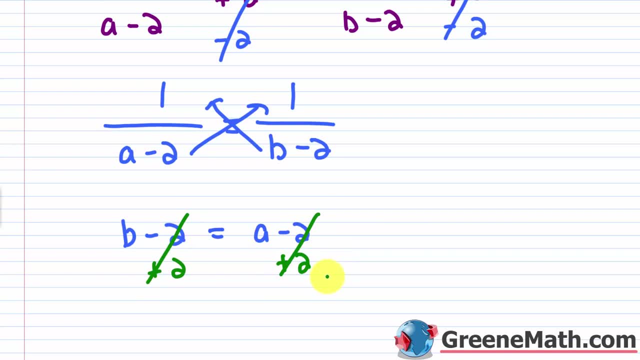 both sides of the equation. this is gone. this is gone, and what I get is that b is equal to a, or you could say a equals b. it doesn't really matter, but you've proved that this is a one-to-one function. So here's the graph, and this one is a bit confusing. 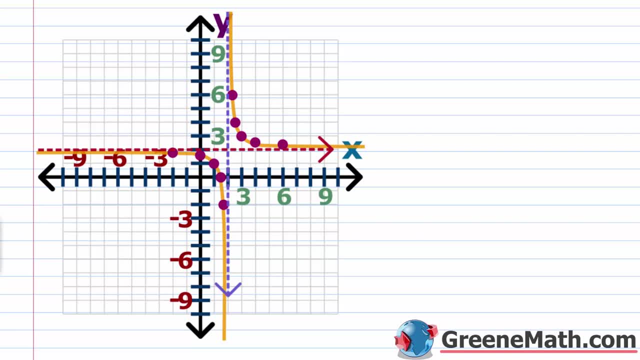 because you do have that horizontal asymptote at y equals 2, but all we're doing here is this graph: if I'm going to the left, it's approaching a y value of 2, but it's never going to actually touch it. This guy is constantly getting closer and closer to 2, but the value isn't always the same. 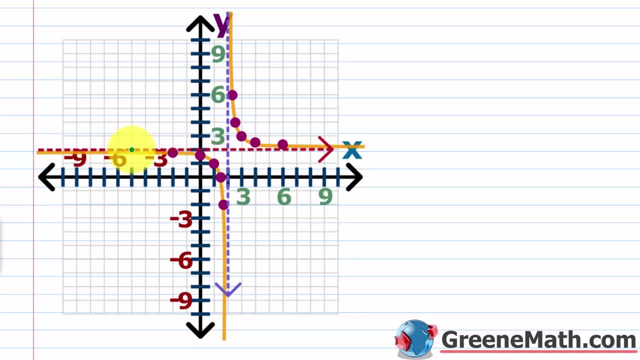 right, it's getting closer and closer. It looks like it graphically because it gets infinitely closer to 2, but it's actually getting closer and closer to 2, but it's actually getting infinitely close to 2 and our eyes, when we look at that, we say, oh, that looks like a horizontal. 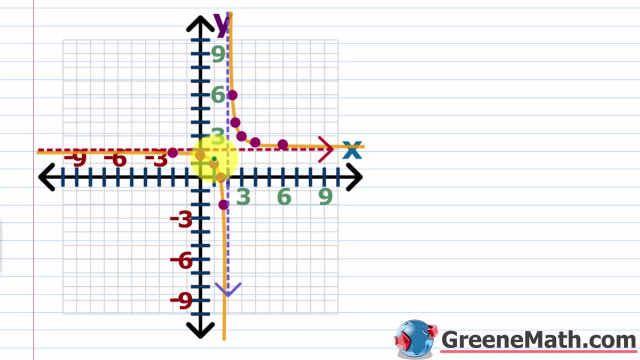 line would hit that in more than one location, but it wouldn't right. so you just have to understand the fact that this is an asymptote and the idea is that it's getting closer and closer and closer. it's not going to actually touch it, but the values aren't the same right? so those y values are. 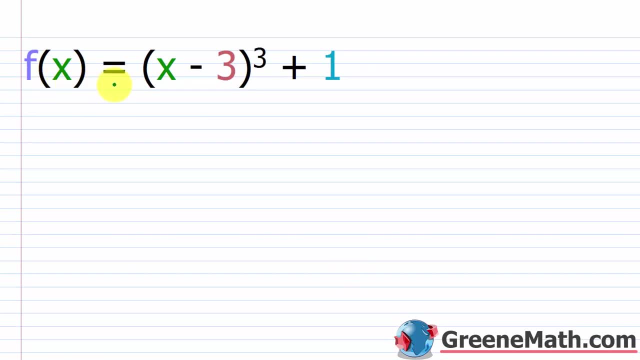 changing. All right, let's look at another one. so now we have f of x equals the quantity x minus 3 cubed plus 1.. So we already know what to do, So we're going to go. f of a is equal to the quantity a minus 3 cubed plus 1, and then f of b. 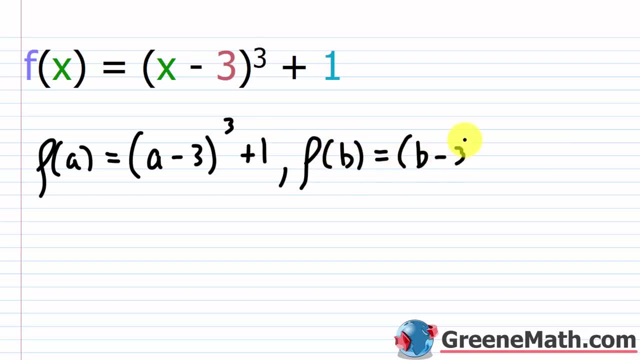 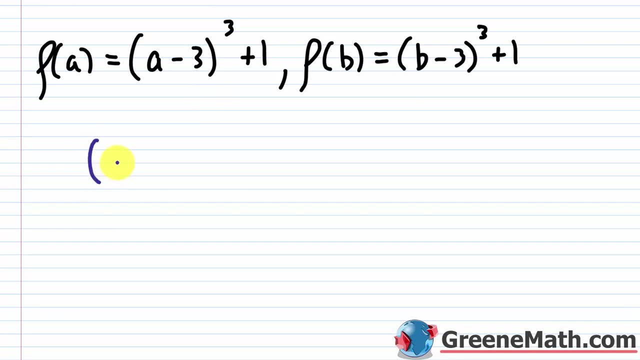 is equal to the quantity b minus 3 cubed plus 1.. Okay, so we're going to set these two equal to each other. so I'm going to say the quantity a minus 3 cubed plus 1 is equal to the quantity b minus 3 cubed plus 1.. So we know that we have one on this side and one on this side. 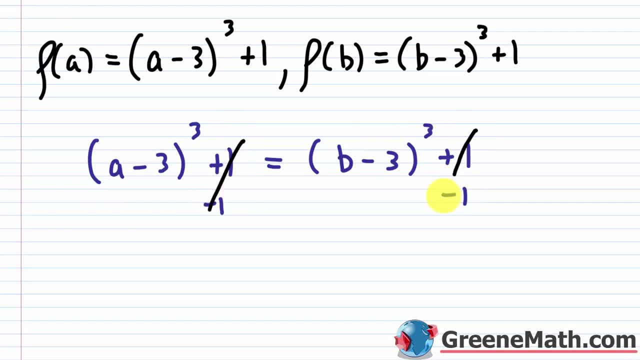 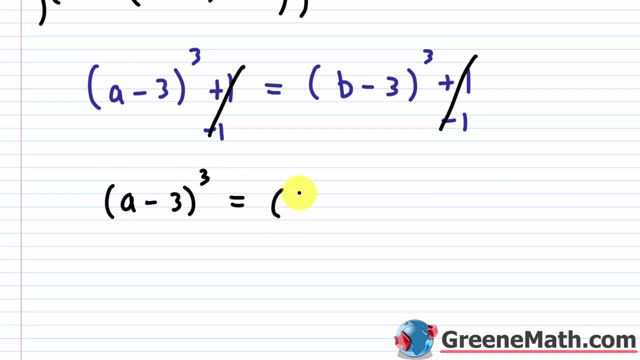 So I can subtract one away from both sides and that's going to go away in each case. So now what I'm looking at is a minus 3 cubed is equal to b minus 3 cubed. Okay, and what I can do to get rid of this kind of exponent of 3. I can use kind of the inverse operation, I can take the cube. 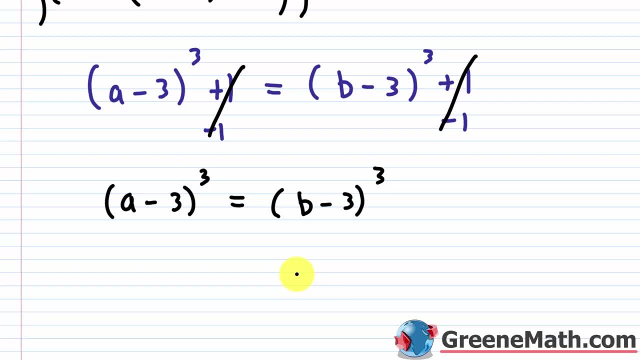 root of both sides of the equation, or I could really raise both sides to the one-third power. It doesn't really matter how you think about that. I'm just going to say I'm going to take the cube root of both sides of the equation, and so we know that this index is going to cancel with this. 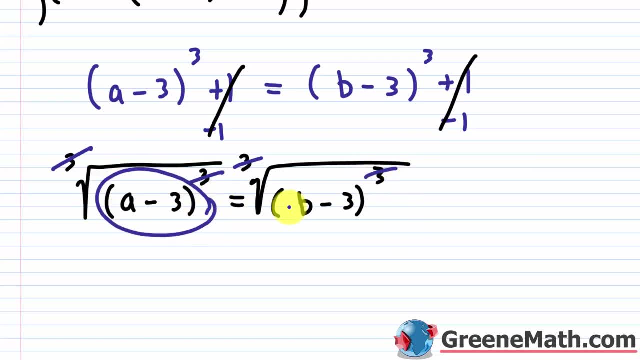 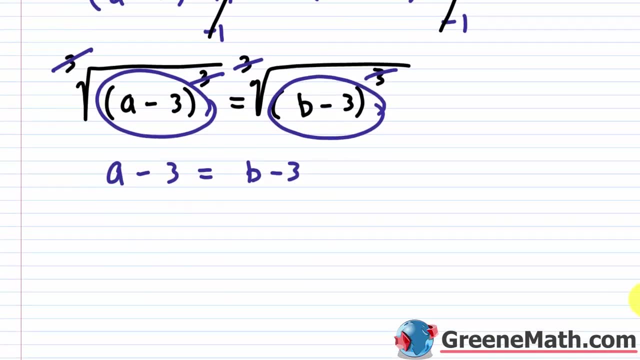 exponent in each case, and that's going to leave me with just this part right here. Okay, so I'm going to have that a minus 3 is equal to b minus 3, and let's scroll down a little bit and we can add 3 to both sides of the equation and we will have that a is equal to b. So a is equal to b.